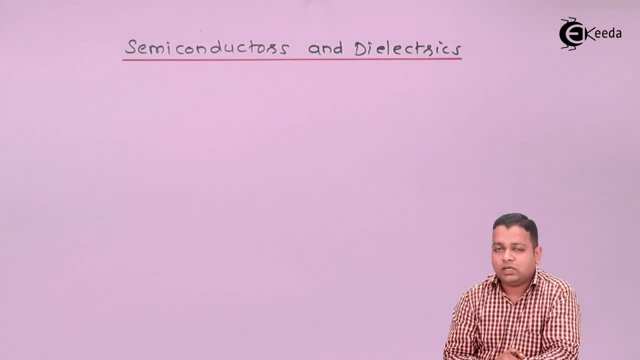 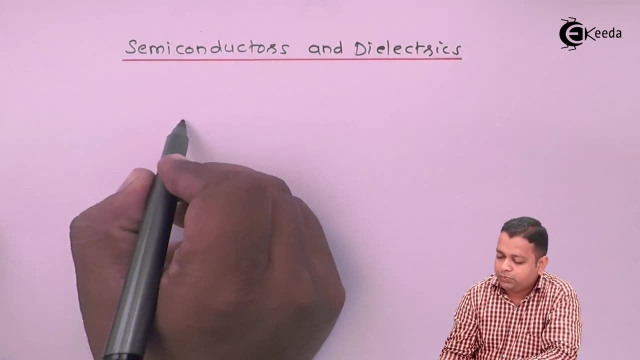 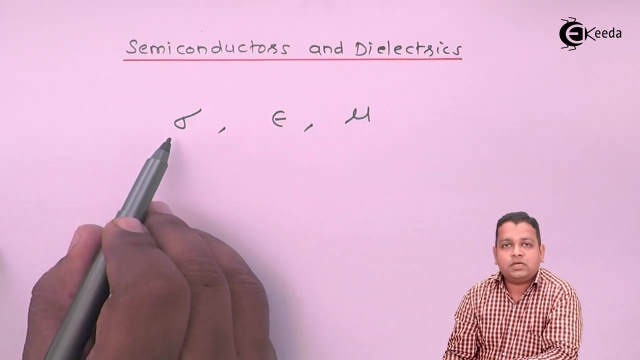 In our subject, electromagnetic field theory generally, the classification of materials with respect to the electric field and magnetic field, we do With respect to the three parameters, That is, sigma, epsilon And mu. Sigma represents conductivity of the material, Whereas epsilon represents permittivity of the medium. 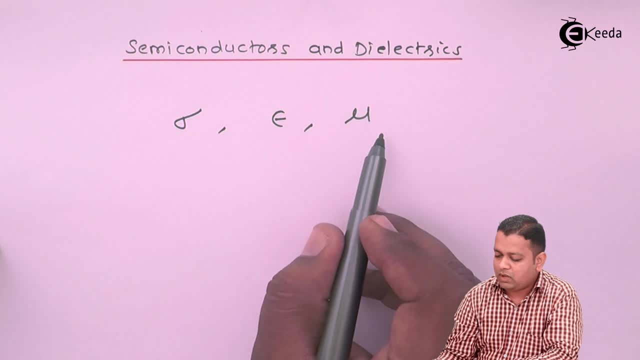 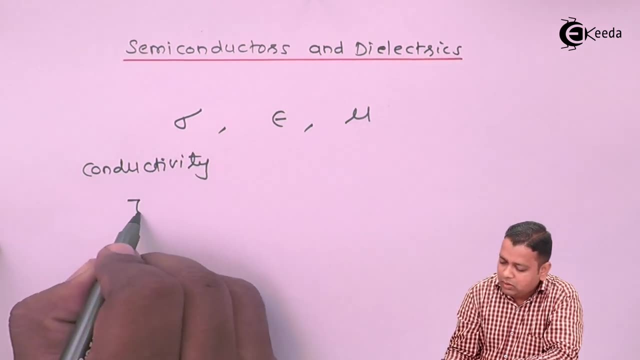 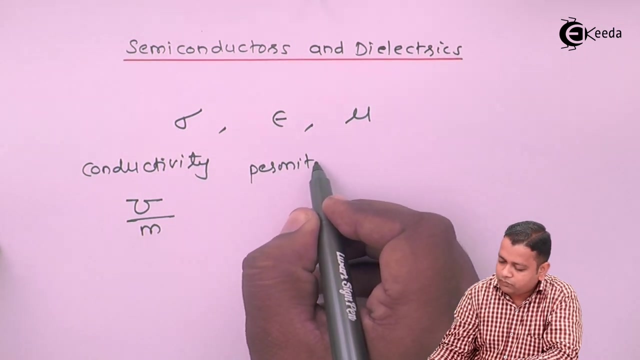 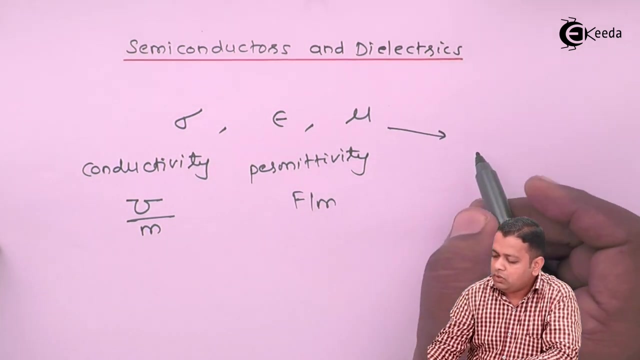 And mu represents permeability of the medium. I here write the names. This is conductivity, measured in mu per metre, Whereas epsilon is permittivity, Permittivity measures measured in parrots per meter and mu. mu is permeability: permeability of the medium measured 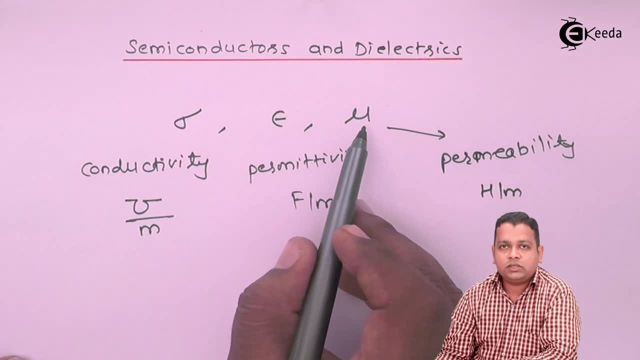 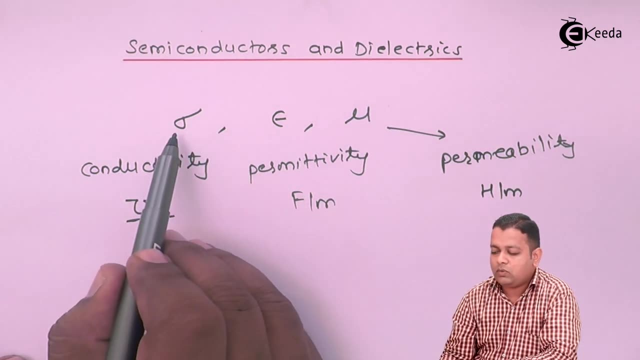 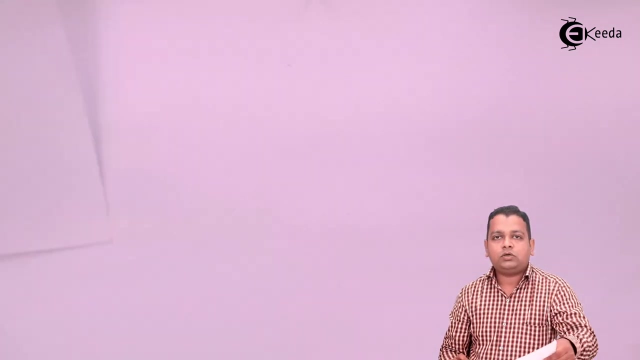 in henry per meter. So mu will be discussed later on in the chapters relating to the steady magnetic fields. Here we will be discussing the conductivity and permittivity of the medium for semiconductors and dielectrics. Now in the topic conductors, properties and boundary conditions, we are well familiar. 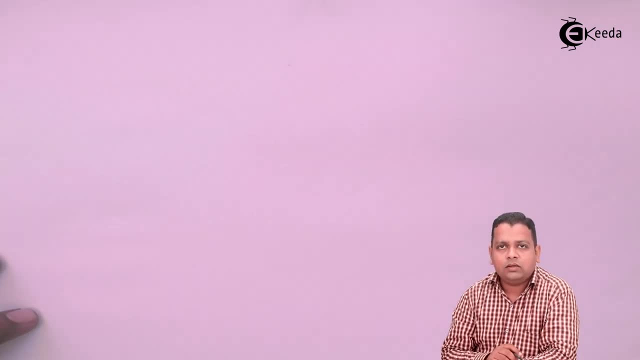 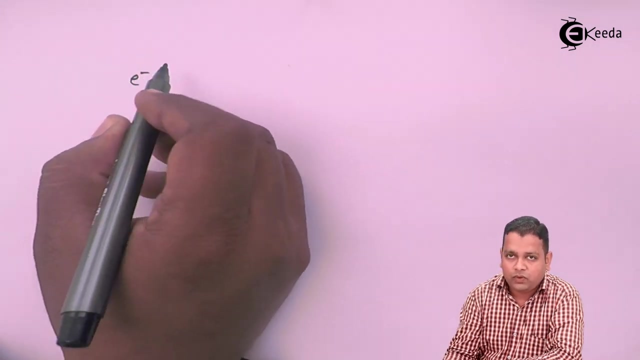 with the relation of conductivity and drift velocity, the charge density. So for semiconductor materials also we require the relationship of the conductivity with the charge densities. Now for semiconductors there are two types of charge carriers, namely negatively charged electrons And positively charged holes. I represent like this: 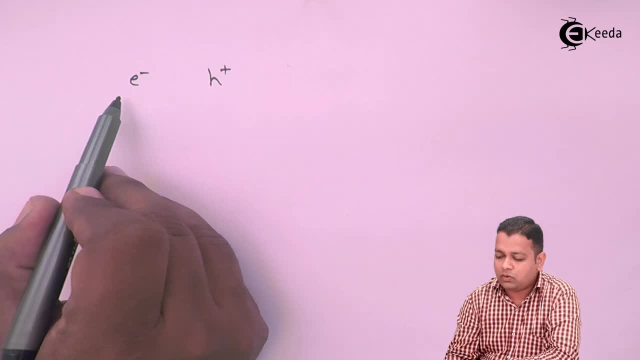 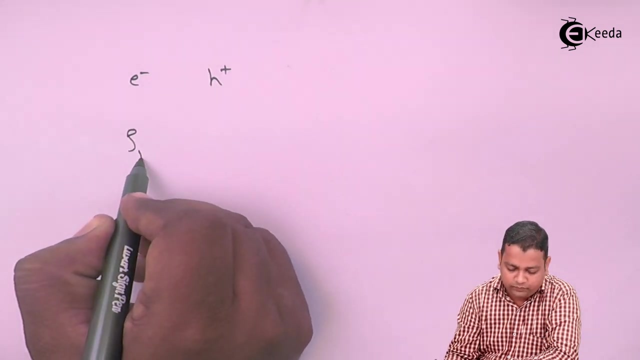 Now, because of the presence of negatively charged electrons and positively charged holes, the concentrations of the electric charges we have to consider along with the charge densities. So let us denote the charge density of electron by rho: suffix, Ve. it is volume charge density of the electron. 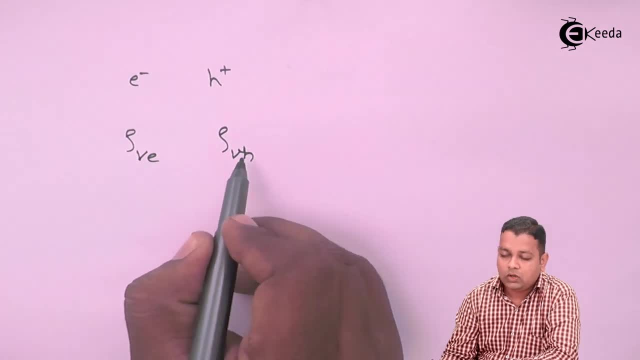 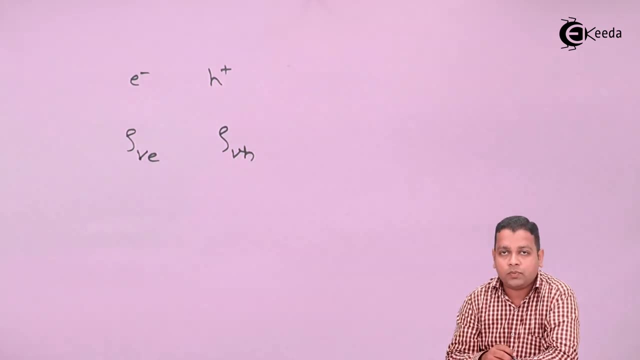 And for the holes rho, suffix Ve. So this is the charge density of the electron, And for the holes, rho, suffix Ve. Now the corresponding mobility of the charges are also to be considered. Hence I represent mu suffix E for the representation of mobility of electron in the semiconductor. 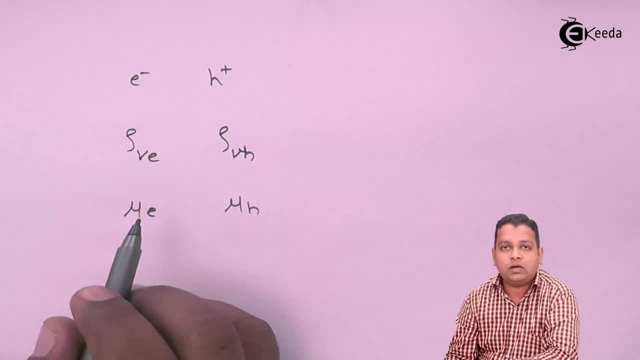 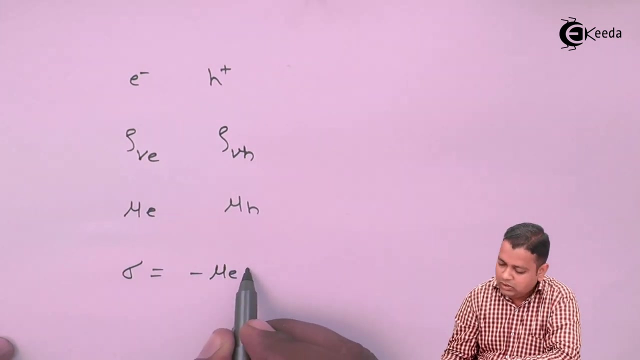 material, whereas mu suffix H represents mobility of holes in the semiconductor materials. As we have seen the relationship in the topic conductor properties and boundary conditions. Boundary conditions: here the total conductivity of the semiconductor shall be given by the relation. Sigma is equal to minus. mu suffix e into rho suffix V. 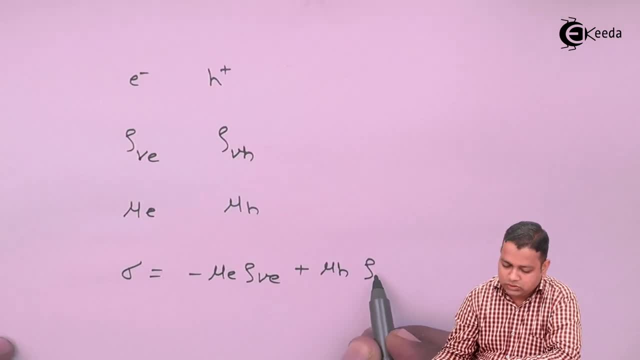 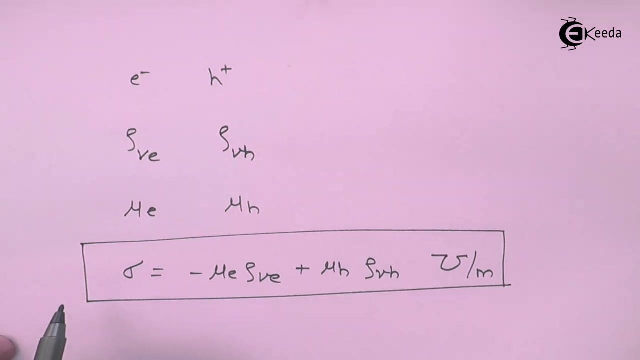 plus mu, suffix H into rho, suffix V, H. as Conductivity is there, We have to put the unit that is move per meter. This relation is very, very important to us to solve two numericals based on to the semiconductor concepts in electromagnetic filtering. Here we have two terms in the right hand side. 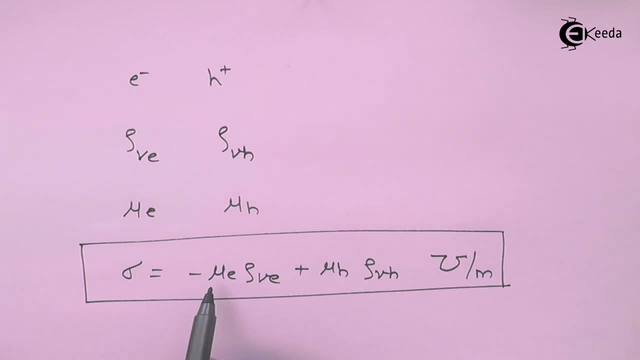 The first term is given the negative sign because the charge carrier is negatively charged electron. here we have the multiplication of Mobility of the charge carrier electron, with the charge density with respect to the volume. similarly, for holes also, We have the product of Mobility of holes with the volume charge density of the holes. 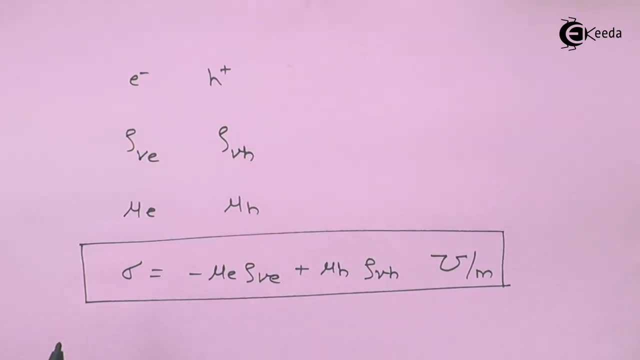 So this gives us the conductivity term for the semiconductor materials. Further, talking about the dielectrics, as We have seen that in metallic conductors the free charge carriers are mostly the electrons and are readily available To us. now in semiconductor We have to give some external source of energy. 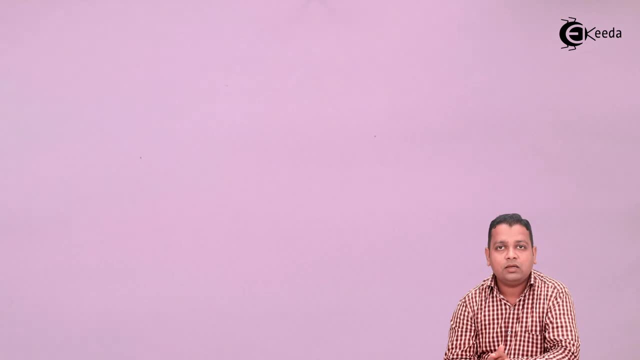 To have formation of charge carriers like electrons and positively charged holes. now in dielectrics. What dielectric materials? or let us say perfect dielectric? the conductivity is zero Because in perfect dielectric mediums there are no free electrons to carry the current. So, as in the dielectric material, we don't have any kind of free charge carriers. 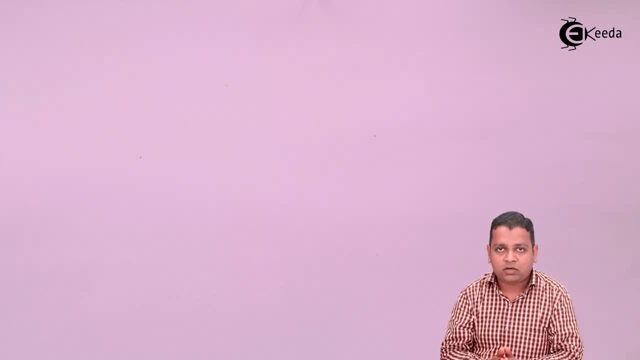 So let us check the conductivity of the dielectric material By placing the dielectric material in certain electric field. if we apply certain electric field to the dielectric material At atomic level, we find that whatever the positive amount of charge will be there that will try to get shifted in the direction. 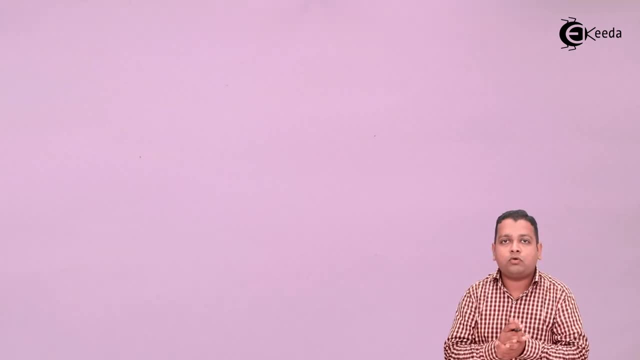 Of the electric field, whereas whatever the negative amount of charge will be there in the material, That will try to get shifted in the opposite direction of the applied electric field. hence this Shows us the formation of electric dipole at atomic level. We have seen the concept of electric dipole in one of our last chapter. 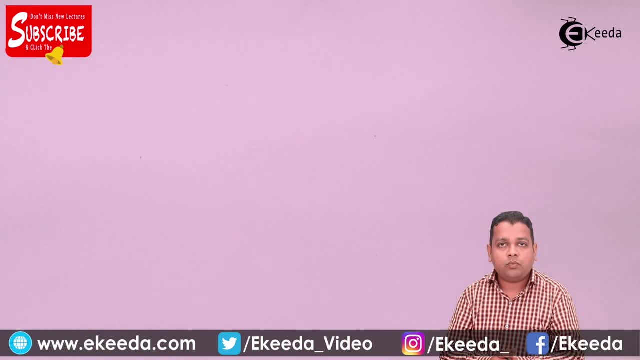 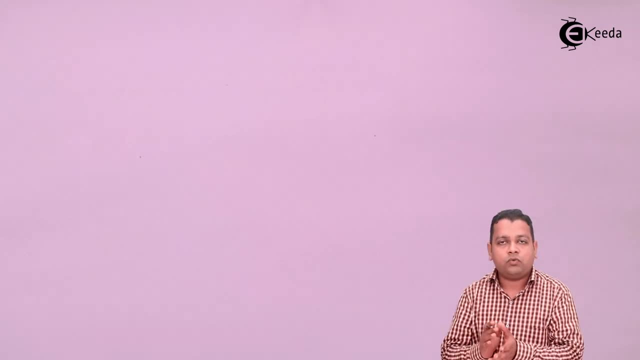 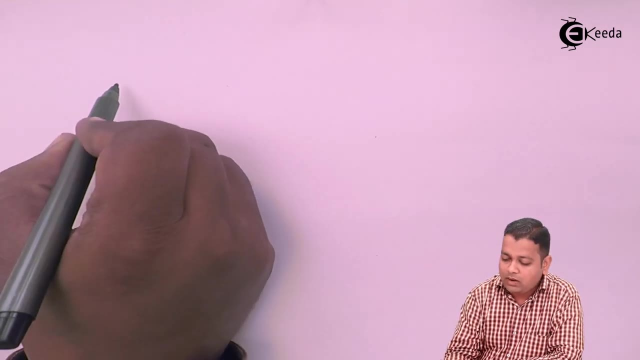 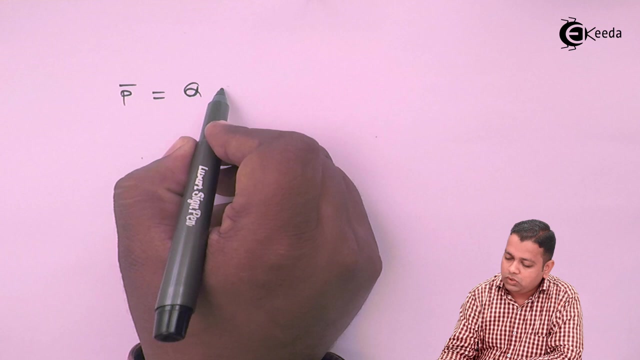 now for electric dipole. the concept of dipole moment also we have seen, which will be convenient to us for analyzing the electric dipole performance in the electric field. So electric dipole moment at the atomic level we have represented by small t bar, given by Q into. 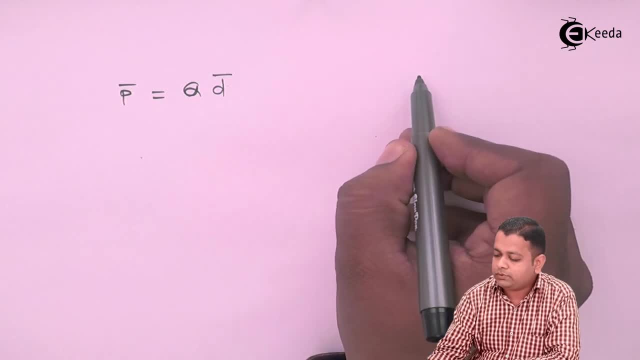 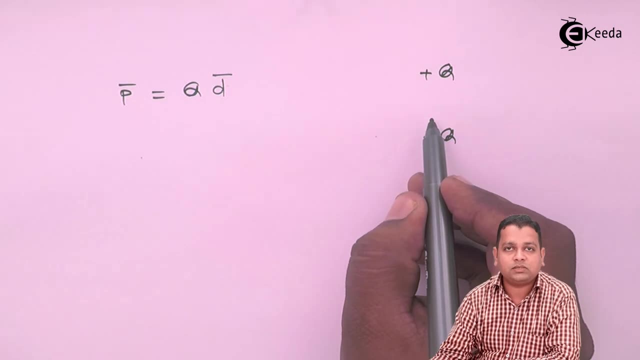 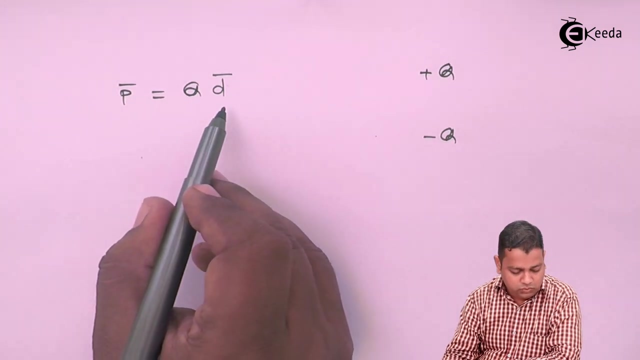 D bar. so d bar is the distance of separation for Positive charge to negative charge. this distance of separation is very, very less as compared to the distance from the source to the field point. Now, t bar is equal to Q times d bar, and Q is the magnitude of the two. 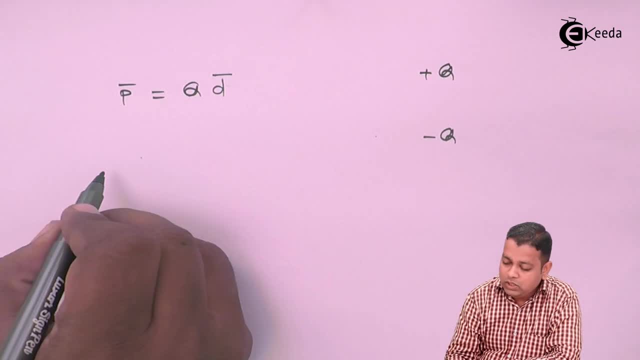 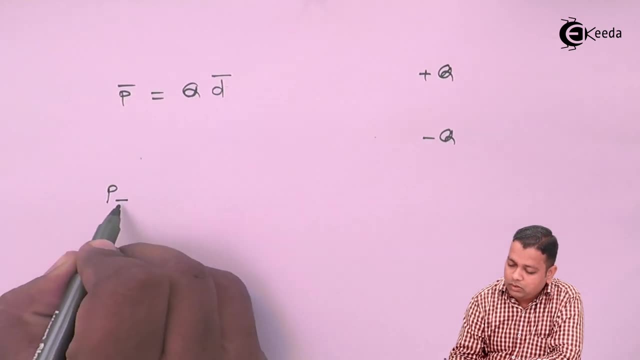 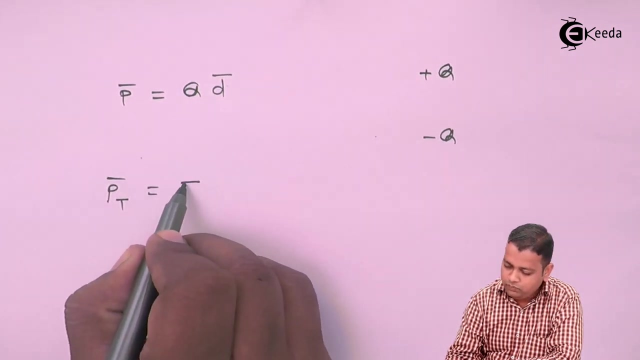 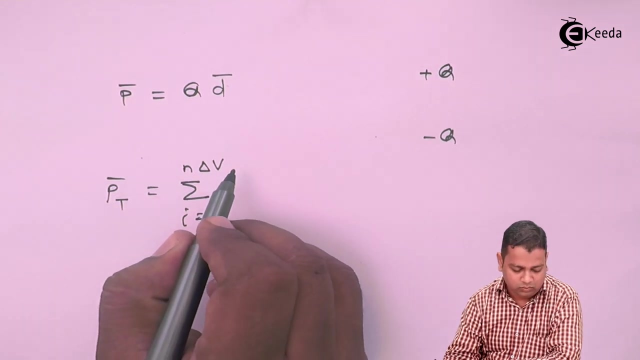 Charges that are having the same value. Now, if there are n number of atoms in the unit volume, so that time the total amount of Dipole moment shall be represented by small p sub x. t bar is equal to Summation. I is equal to 1 to n times Delta V, the incremental volume. 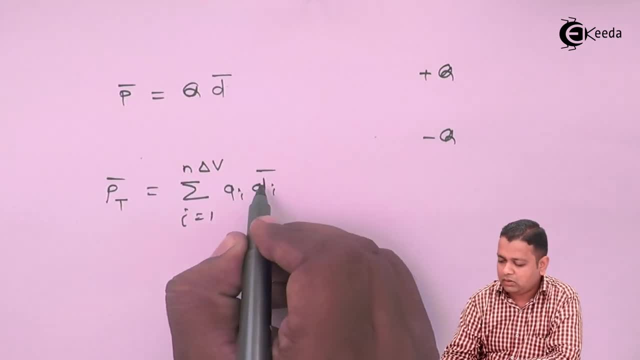 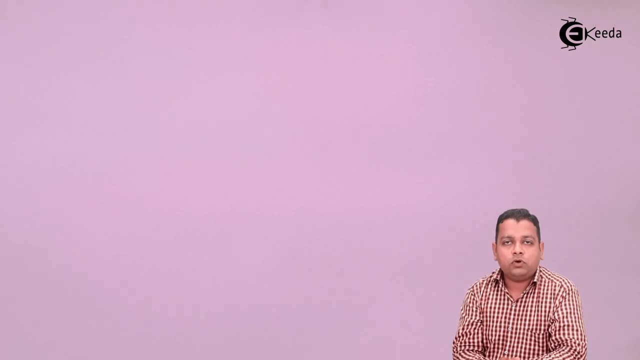 Q sub x i, D sub x i bar. so Q i is the i-th Atomic dipole charge. so from the term dipole moment, what we have seen for electric dipole, for the entire dielectric material under consideration, We have to see the new term which is derived from dipole moment, called as polarization. 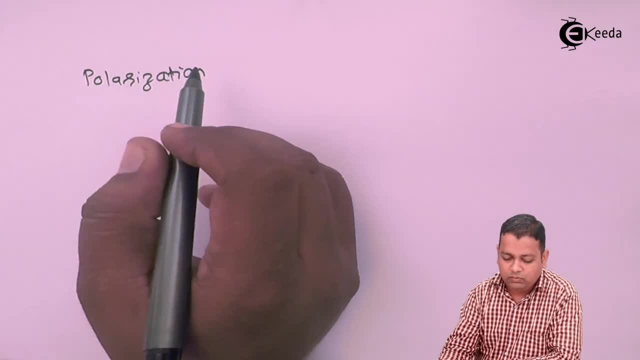 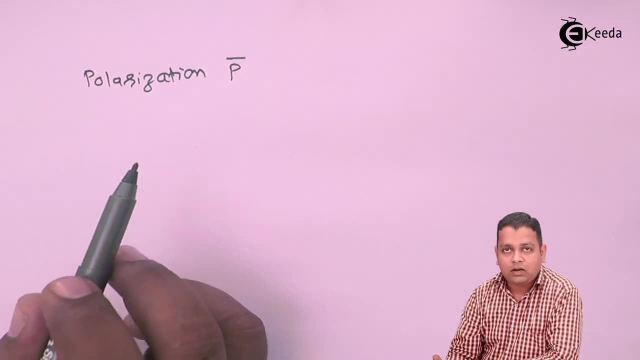 So the term polarization is a vector term and it is represented by capital P bar. the term polarization is for the entire dielectric material and defined as the total Dipole moment per unit volume at the point in the dielectric Hence we can represent the dipole. 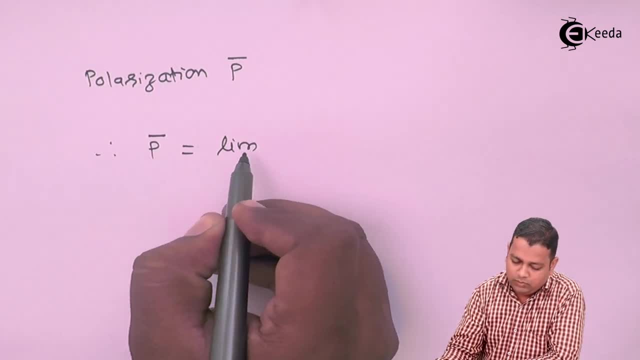 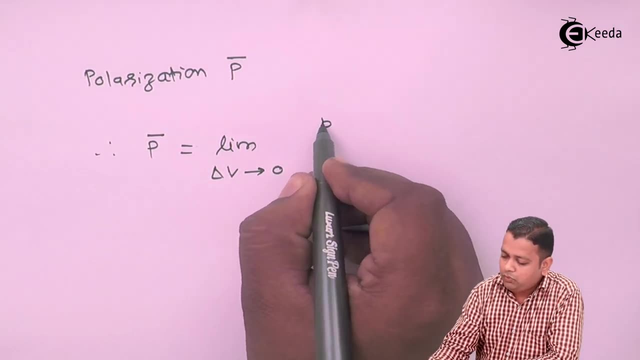 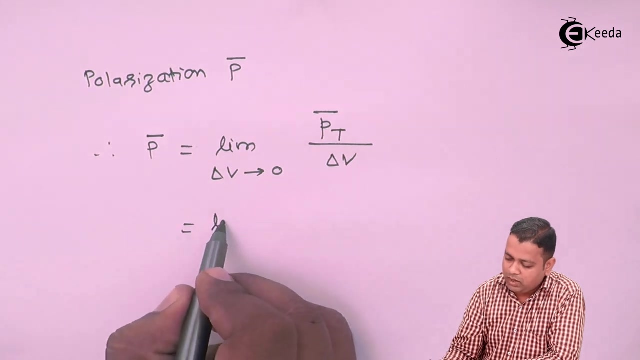 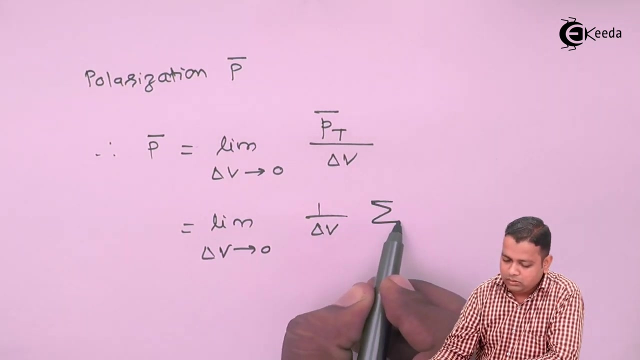 Polarization capital. P bar is equal to limit. Delta V, which is incremental volume, tends to 0. the total dipole moment represented by small p sub x, t upon delta V. so it shall be given by limit: Delta V tends to 0, 1 upon Delta V. here we have the summation, that is, I is equal to I. 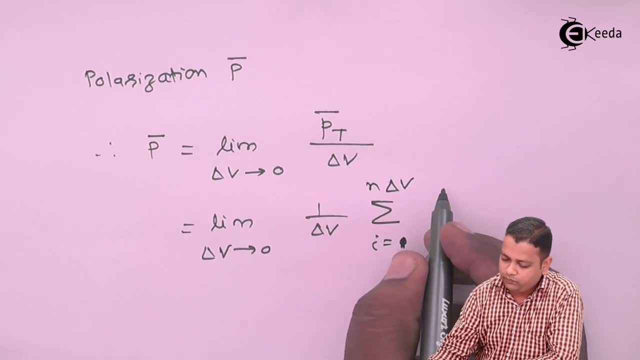 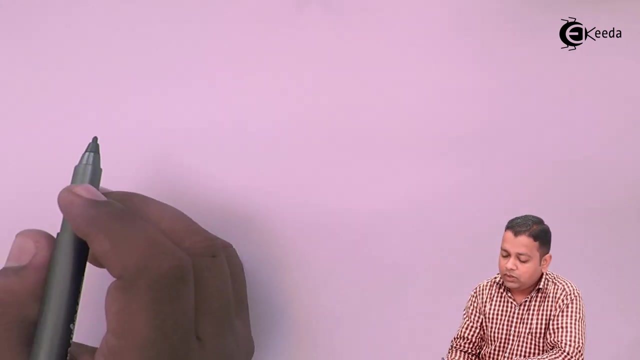 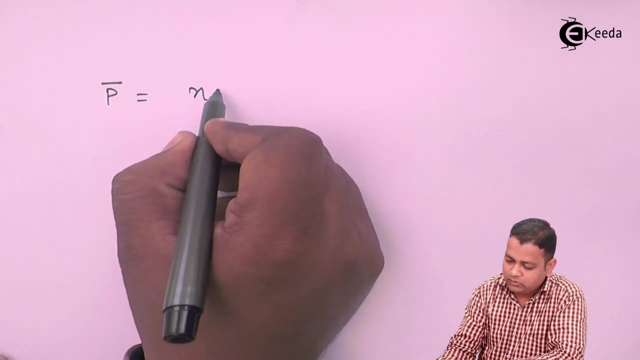 Is equal to 1 to n times Delta V Dipole, moment of Ith dipole in terms of Coulomb per meter square. So if all the dipoles in the dielectric material are identical, then we can write the polarization term. capital P bar is equal to that is N times Q D bar. 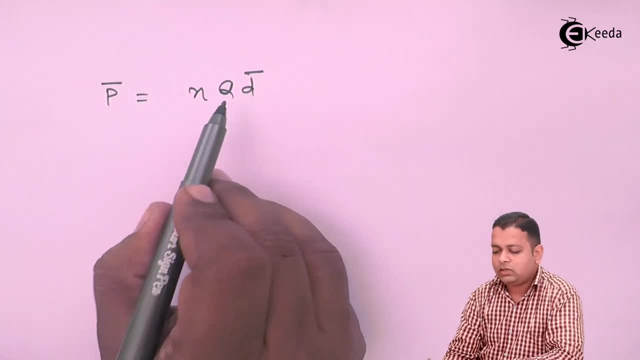 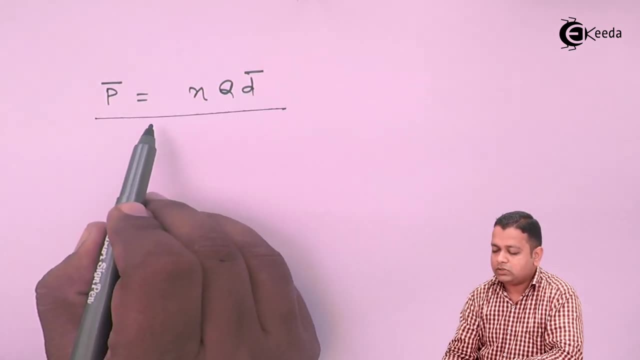 Okay, so Q D bar is the dipole moment for one electric dipole. so for M electric dipoles into the dielectric material We can have, P bar is equal to N times Q D bar. N Q Q times D bar is dipole moment. 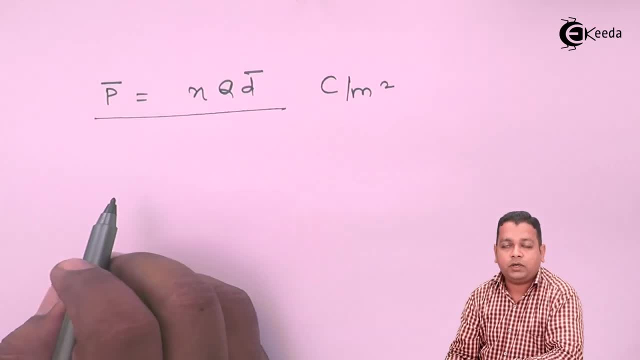 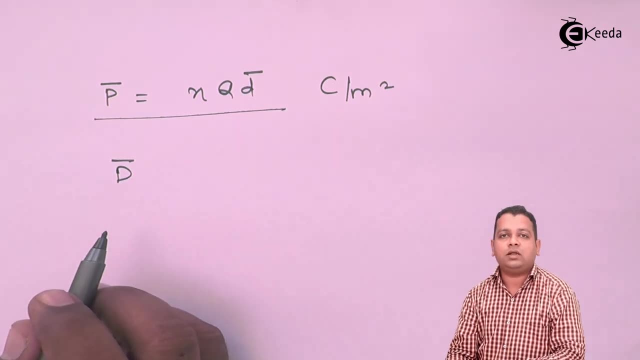 So the unit we have to provide- Coulomb per meter square, now Now pulm per meter square- is the unit we have generally given to D bar, which is called as electric flux density. for the charges, whatever the flux lines are emerging out with respect to the area crossed, we have defined the term electric flux density. 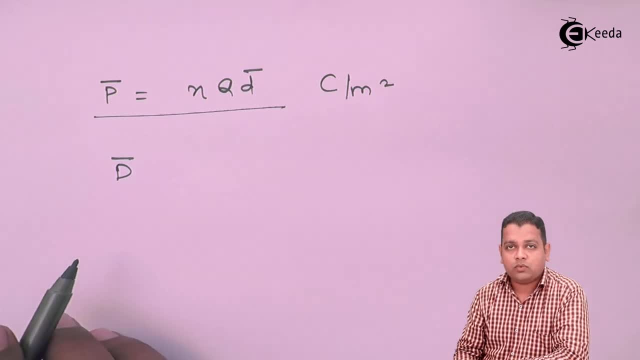 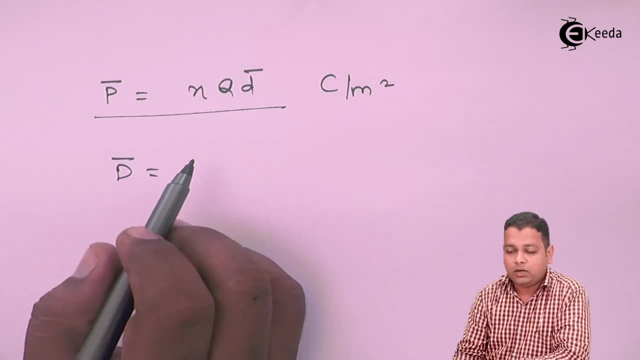 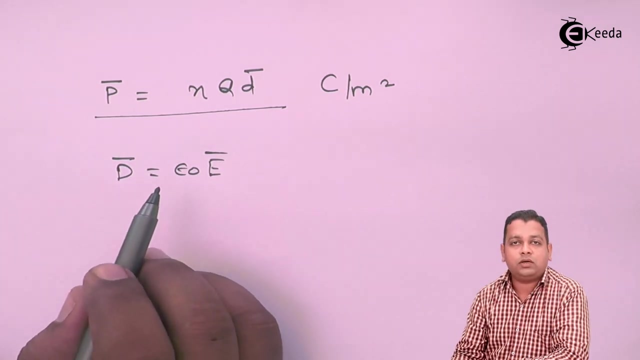 Now in chapter number three, electric flux density, bosses, law and divergence, we have seen the relation of electric flux density for the point charge with electric field intensity. by this relation, D bar is equal to epsilon 0 E bar when the charges were considered to be placed in the free space. 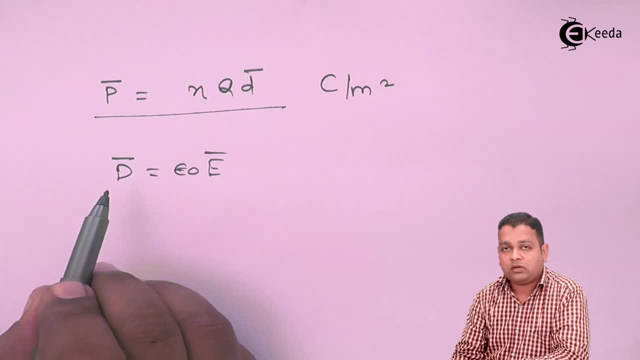 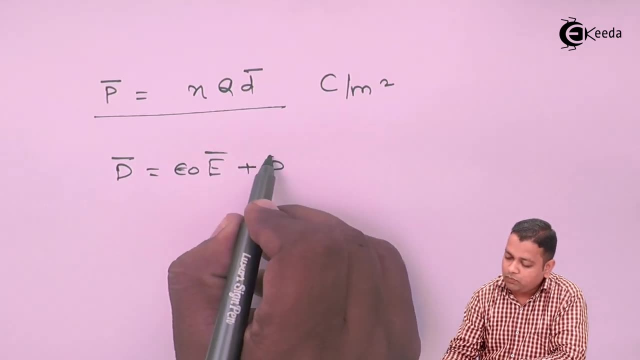 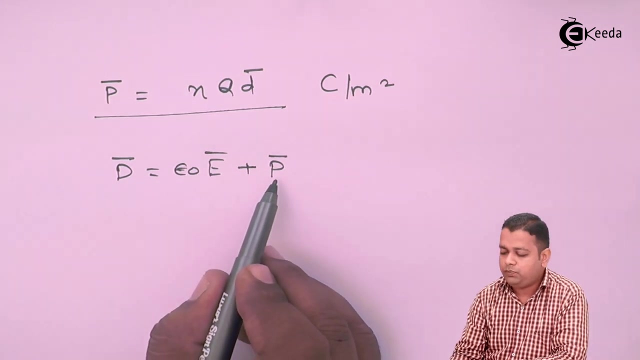 Now if the medium is any dielectric medium, so that time we have to modify this relationship, we have to add for any dielectric medium its polarization term. So D bar will be equal to epsilon 0 times E bar plus P bar. that is polarization for. 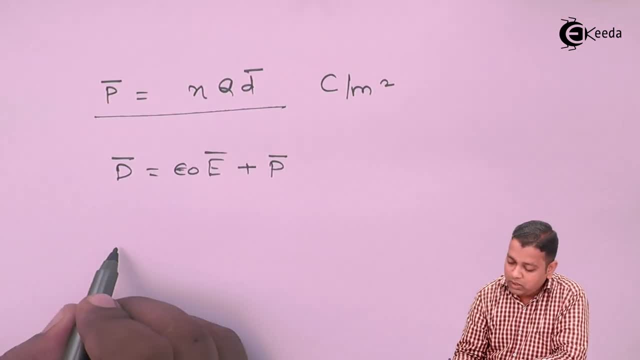 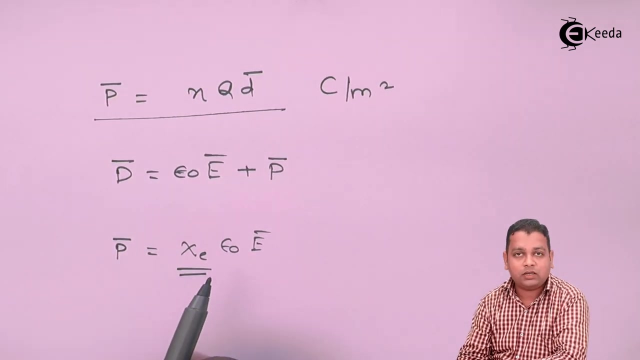 the polarization. Now this polarization term is having relationship with the electric field intensity given by the relationship that is, x E epsilon 0 times E bar, where this term is called as susceptibility of the dielectric material, which indicates the how much dielectric can be polarized in.